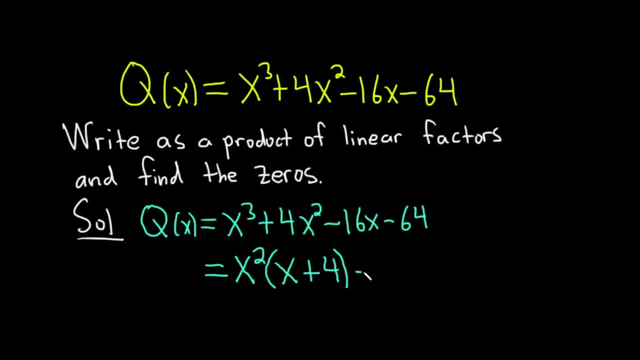 a negative and a negative. So let's go ahead and try to pull out a negative 16.. And then parentheses. And so here we're missing an x, because negative 16 times x is negative 16x. And then here this is going to be a plus 4, right, Because negative 16 times 4. 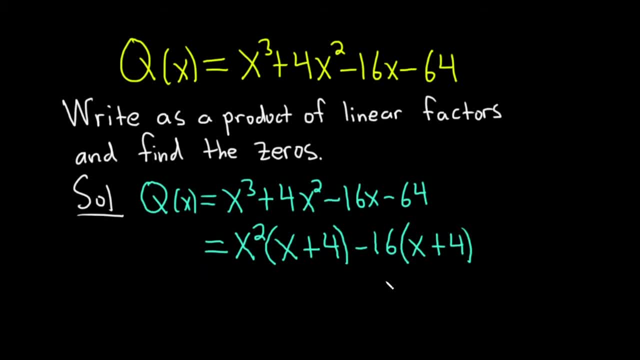 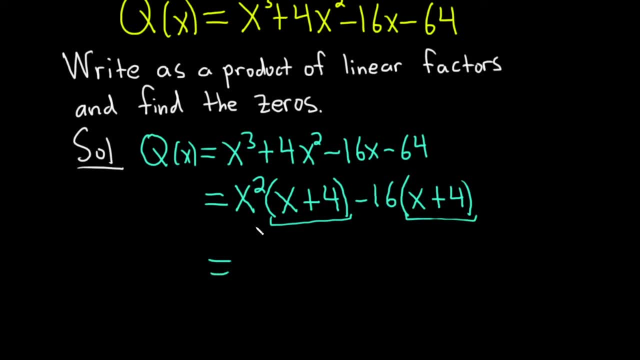 is negative 64.. Okay, So now we can pull out the common factor x plus 4.. And you can put it in the front or you can put it in the back. I'm going to put it in the front. 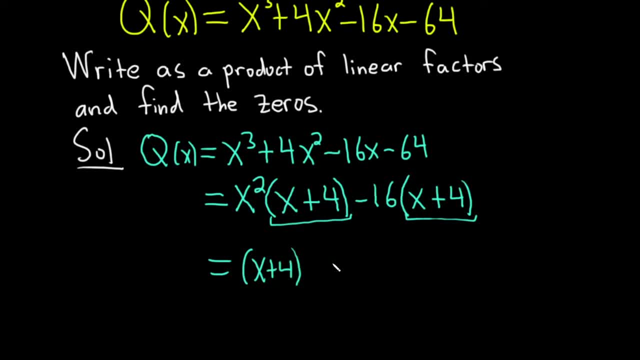 like this: x plus 4.. This looks a little bit cleaner. And then you say: what do you multiply by x plus 4 in order to get x squared times x plus 4?? Well, x squared right Because x plus 4. 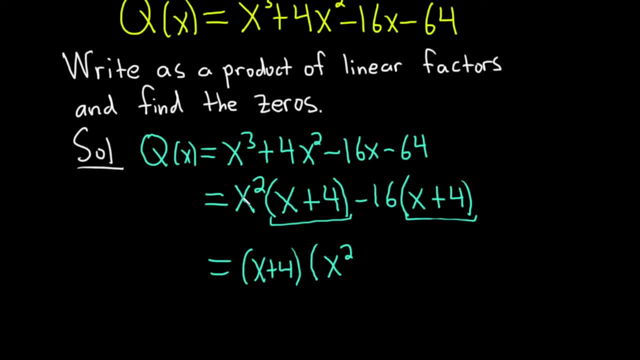 times x squared is x plus 4 times x squared. It's just written backwards, And then here we've already pulled out the x plus 4. So we just have a minus 16.. And again, just a mental check. 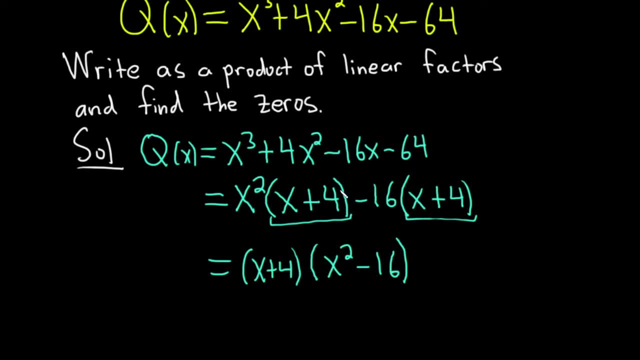 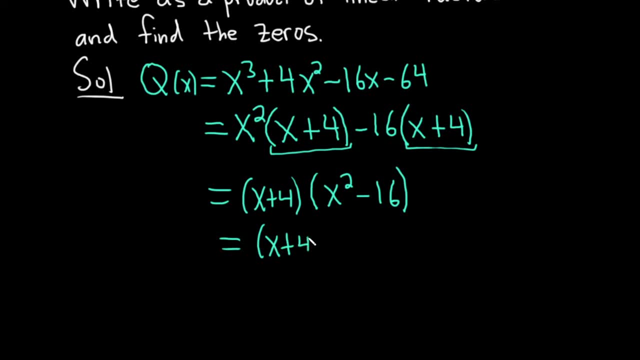 x plus 4 times minus 16.. is exactly what we have here. Let's keep going. This is equal to x plus 4.. This is actually the difference of squares. It's x squared minus 4 squared, So it's x minus 4,. 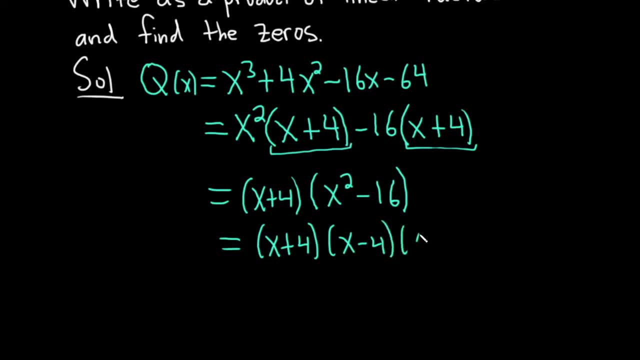 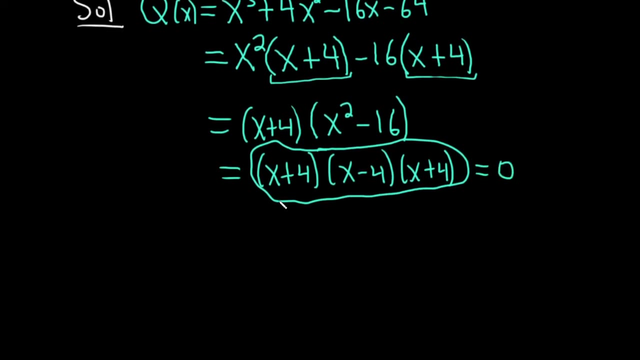 x plus 4.. So x minus 4,, x plus 4.. And we've done it, We've written it as a product of its linear factors To find the zeros. we basically have to find the zeros. So basically set it equal to 0. And then we can see what the answers are right away. Basically, 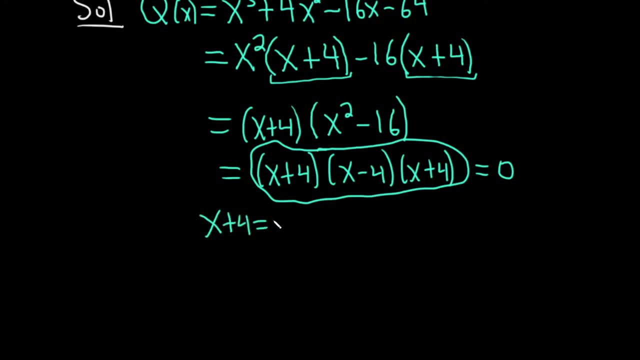 you set each factor equal to 0. after that, if you wanted to, Then x minus 4 equals 0. And then x equals 4.. x plus 4 equals 0. You subtract 4 here, So you get x equals negative. 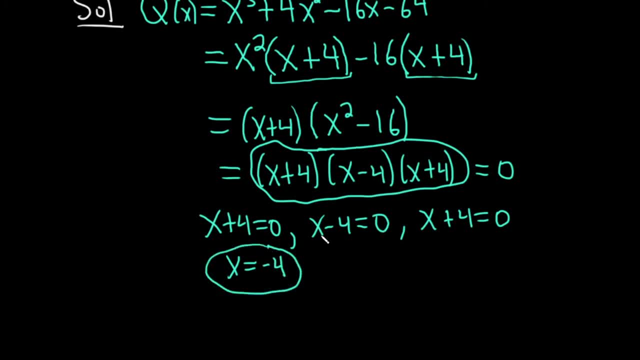 4.. That's one of the answers. You add 4 here, So you get x equals 4.. That's another answer. Subtract 4 here, So you get x equals negative 4.. That's another answer. So you get x equals negative 4.. That's another answer. So negative 4 appears twice In this case.